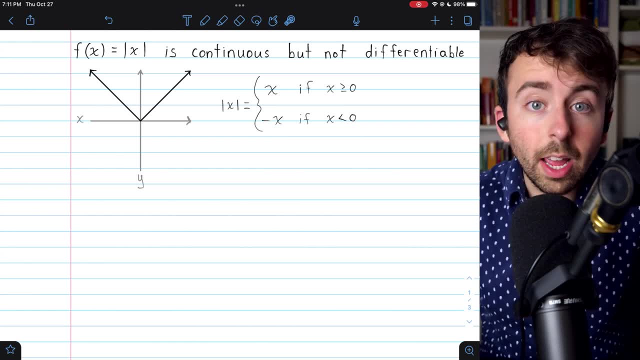 value function is defined- And here is its definition- as a piecewise function. The absolute value of x is Simply x when x is at least zero And the absolute value function is negative x if x is less than zero. since if x is less than zero, the absolute value function will have: 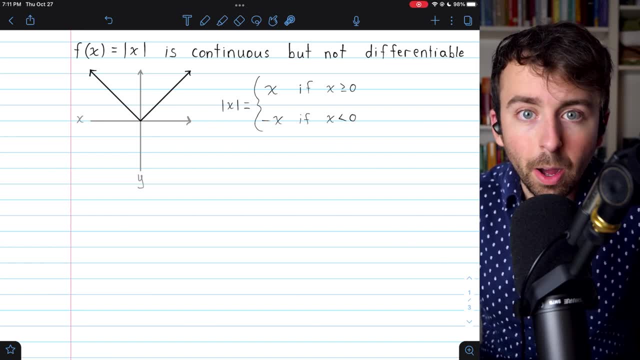 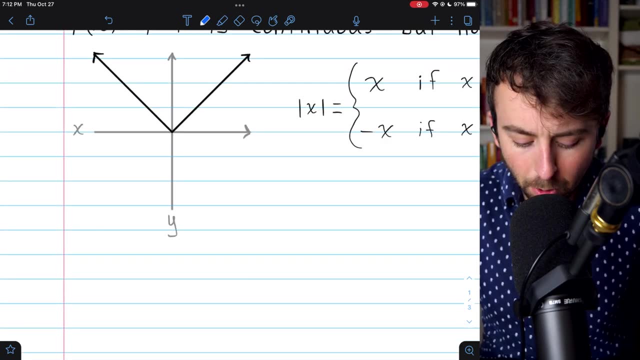 to hit it with another negative in order to make it positive. So if we consider the continuity of this function at any point with an x value less than zero, that would look something like this: Here's a point to the left of zero, Then approaching: 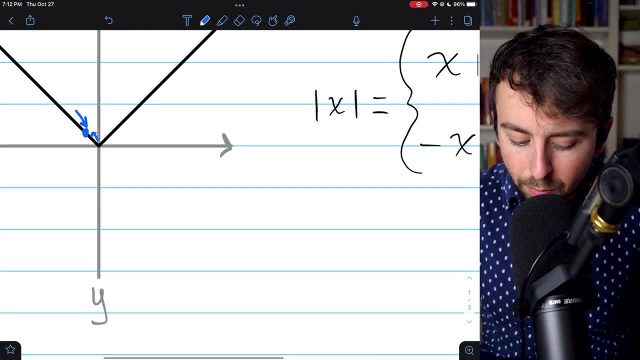 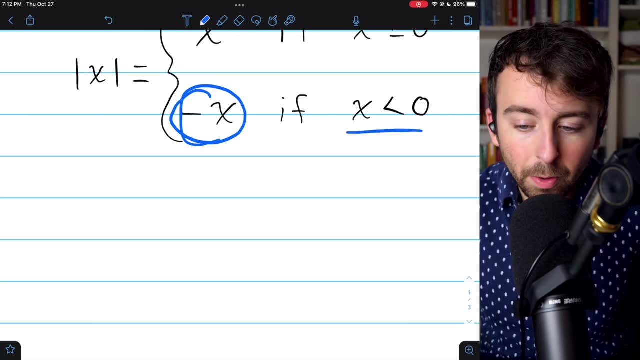 from the left of zero, we have a point to the right of zero And if we consider the from the left and approaching from the right, we just have our function behaving like this: Negative x, because we're talking about where x is less than zero And every polynomial 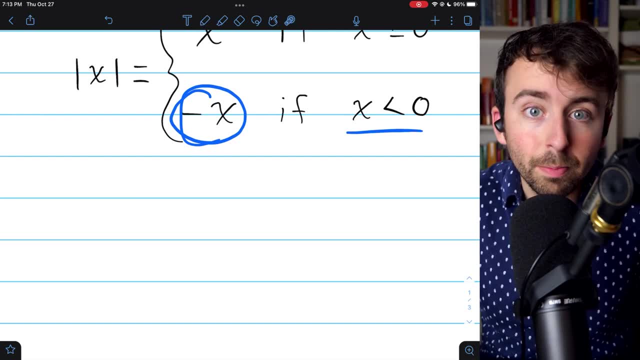 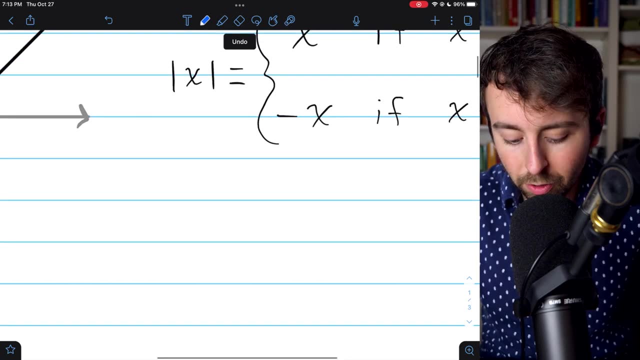 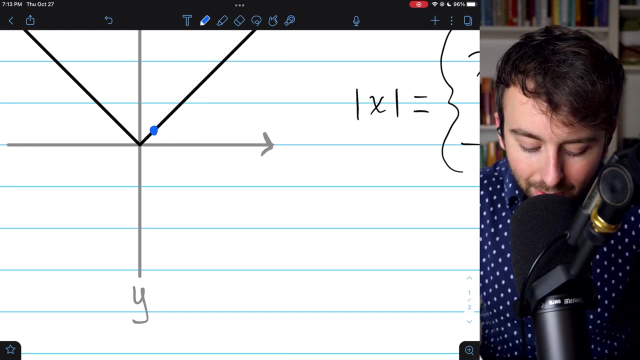 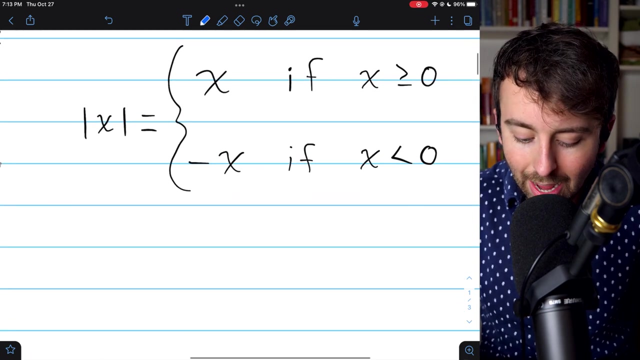 is continuous. Negative x is just a simple polynomial. So certainly, if x is less than zero, well, at all those places the absolute value function will be continuous. Similarly, if x is greater than zero, that would look something like this: Then, approaching from the left and approaching from the right has our function behaving the same way, which is just as x. 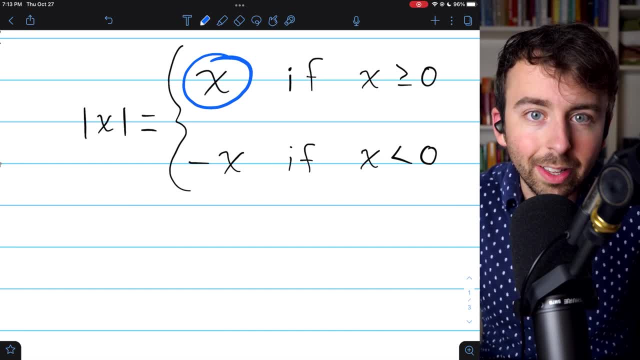 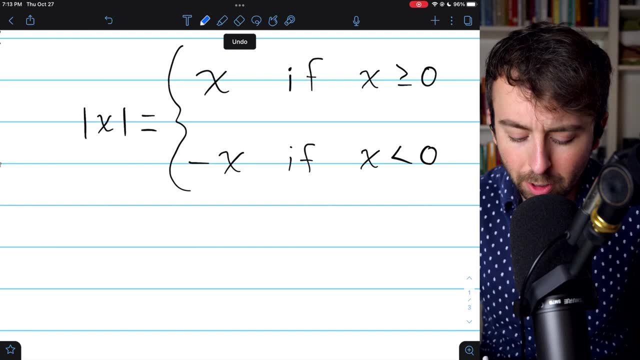 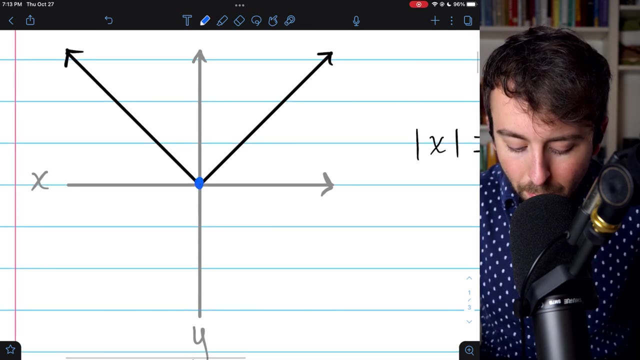 x again, is a polynomial which is certainly continuous. So the absolute value function is continuous for all x less than 0 and for all x greater than 0.. The only point that deserves special attention is where x equals 0, because right here the behavior of the function to the left is different from the behavior from the right. 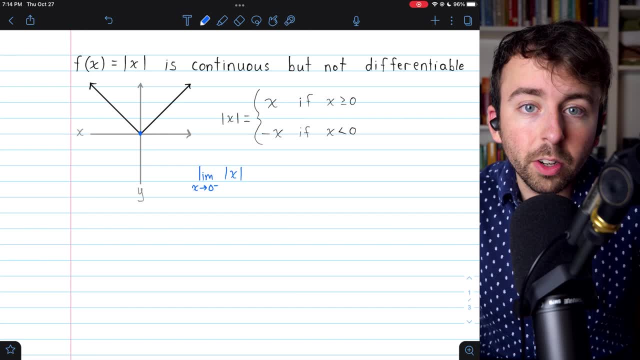 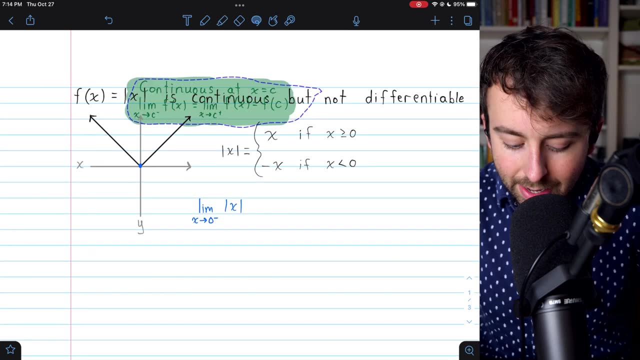 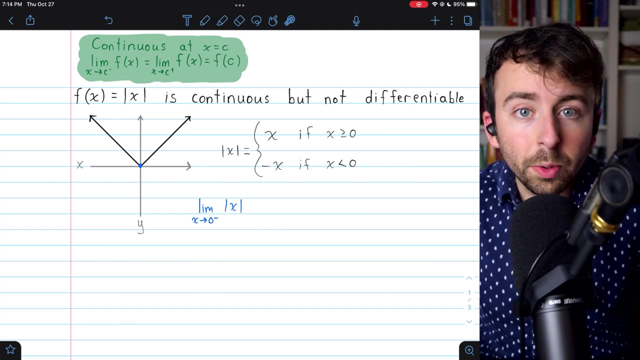 However, we can fairly easily show that the absolute value function is indeed continuous even at this point. x equals 0.. To do that- recall the definition of continuity, In order to show the function is continuous at x equals 0, we'll need to show that the limit of the absolute value function as x approaches 0. from the left. 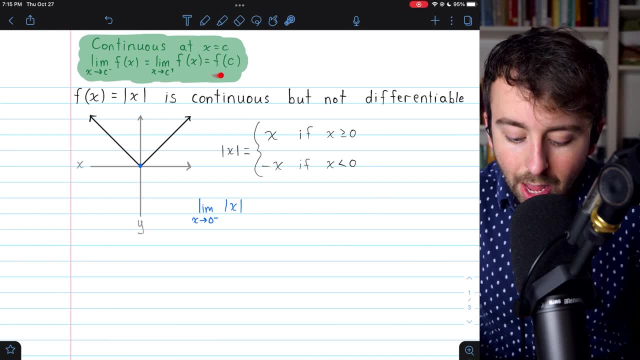 is the same. It's the same as from the right, which is the same as the value of the absolute value function at x equals 0. So let's begin this process by considering the limit of the absolute value of x as x approaches 0. from the left. 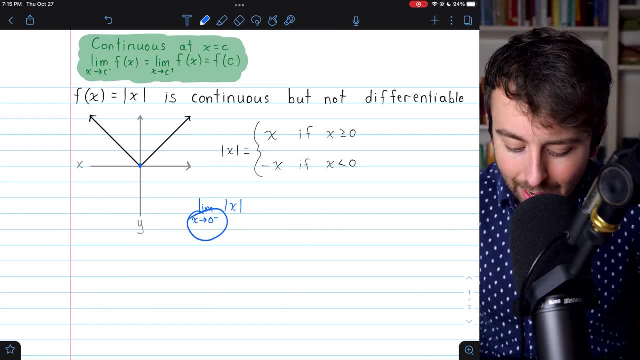 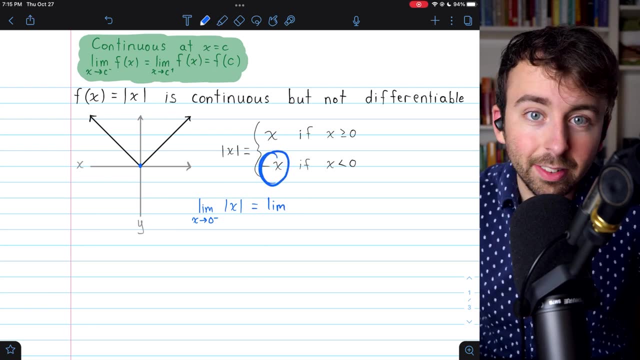 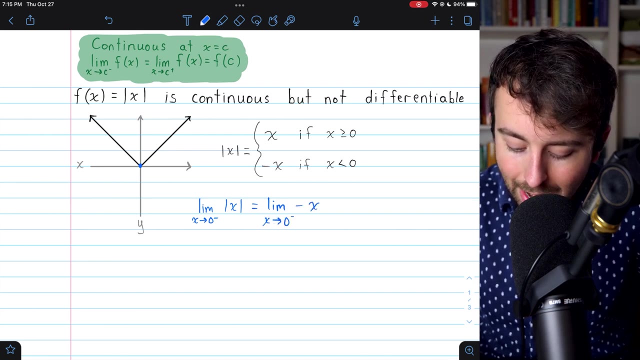 In this situation, since x is approaching 0 from the left, all of the x values are negative. So the absolute value of x will be negative. x in order to flip it and make it positive. So this is the same as the limit, as x approaches 0 from the left, of negative x. 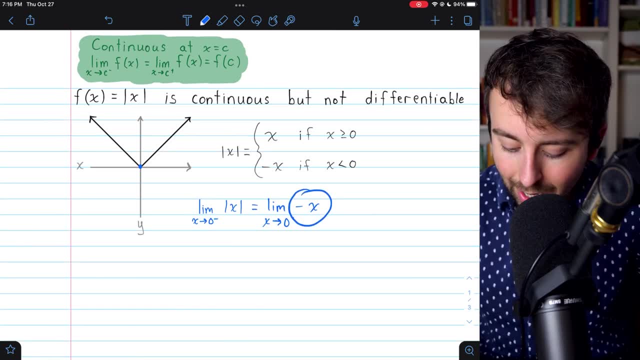 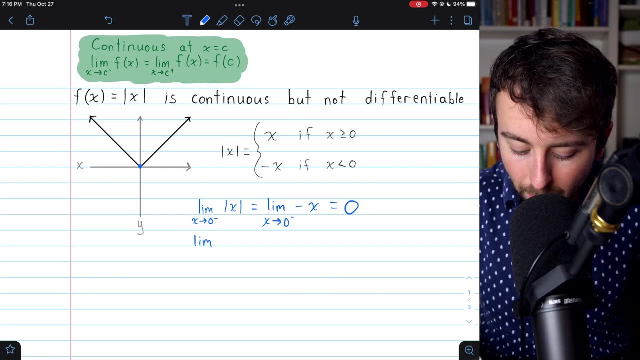 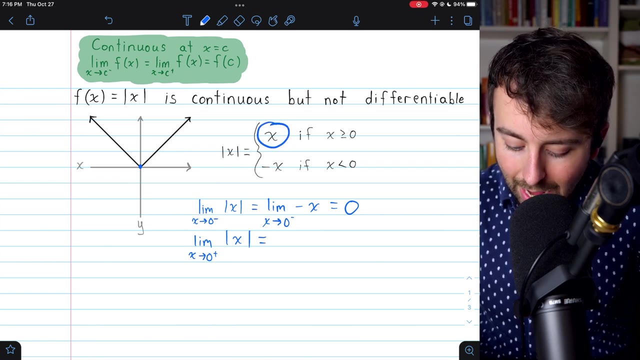 And then certainly we could just plug 0 in to find that this limit is equal to 0.. And a similar thing is true for x approaching 0 from the right. From the right, since all the x values are positive, the absolute value of x is just x. 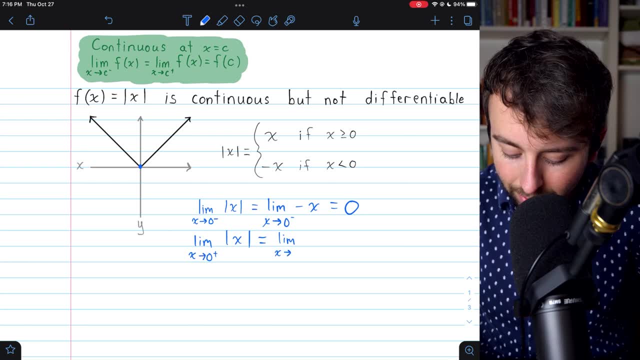 And so this limit is the same as the limit of x approaching 0 from the right, or, excuse me, as x approaches 0 from the right, the limit of x, because absolute value of x is just x. when x is positive Again, we could now certainly plug in 0,. 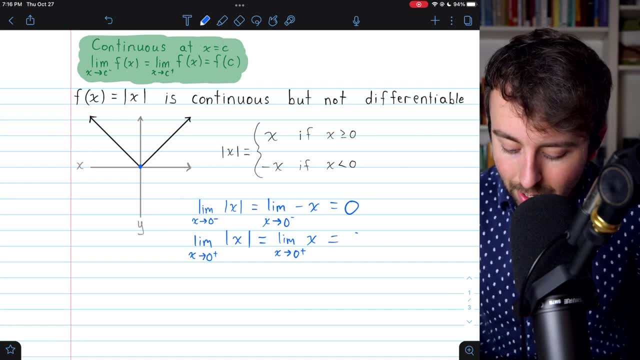 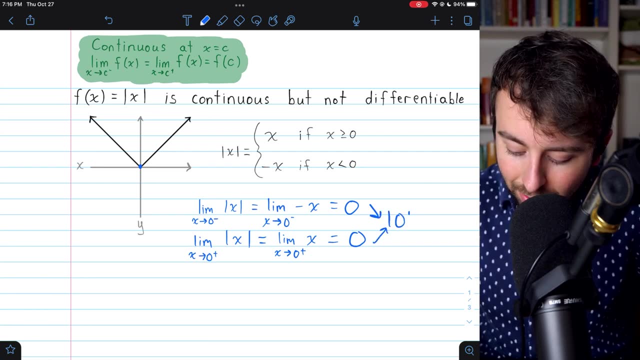 since we know that x is continuous, and this will then be equal to 0. And furthermore, what is the value of the absolute value function at x equals 0?? Well, that would just be 0.. So we see the absolute value function's limit. 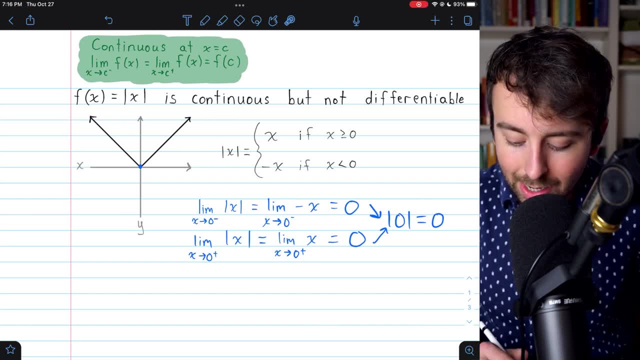 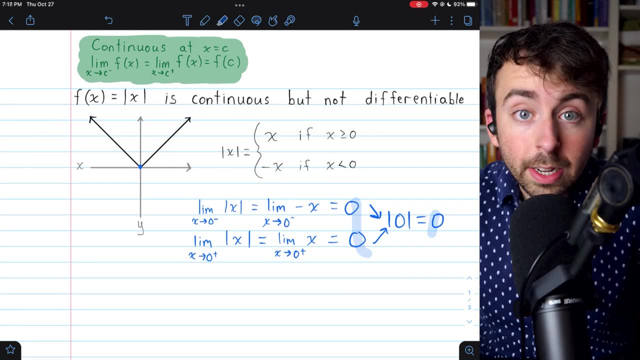 from the left of 0 equals the limit from the right of 0, which equals the value of the function at 0. They all happen to equal 0.. Now we've finished justifying the fact that the absolute value function is continuous on its entire domain. 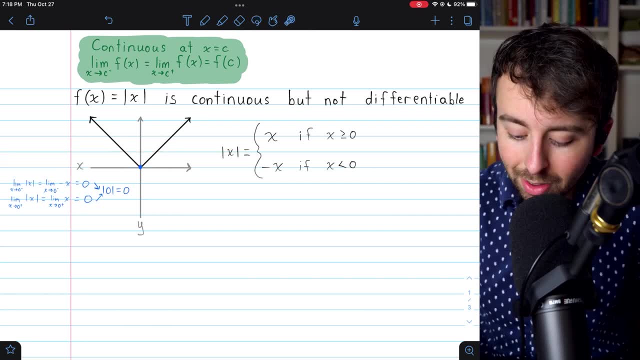 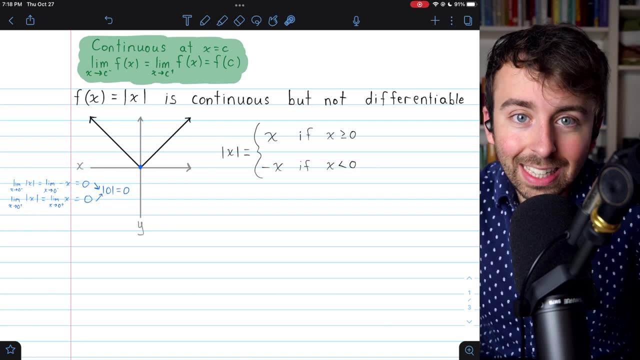 I'll move our work off to the side to make some room to show that this function is not differentiable. It is differentiable at most of its points. If x is less than 0, the derivative would just be negative 1. And if x is greater than 0,? 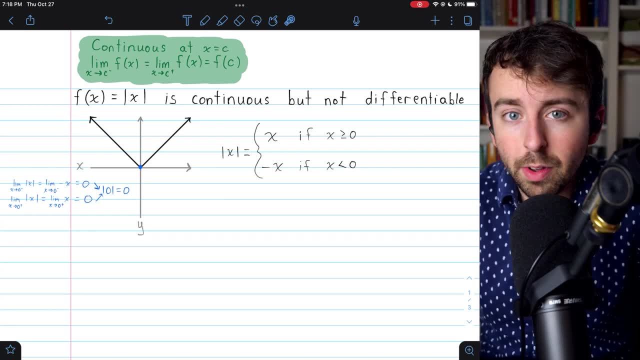 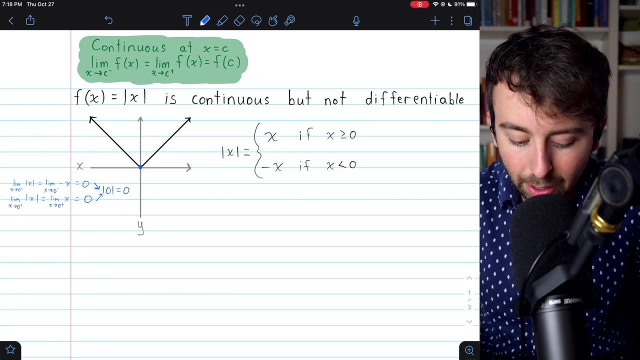 the derivative would just be positive 1.. I'll leave it to you to verify that. I want to spend the rest of the lesson focusing on the non-differentiability of the absolute value function at x equals 0.. It's right here where the function 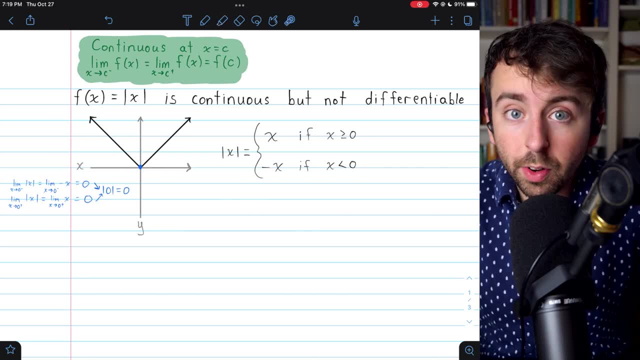 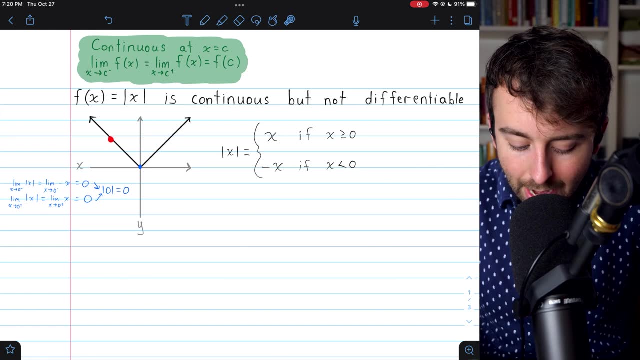 fails to be differentiable. I hope you can see why the function is not differentiable at x equals 0 intuitively from the graph, because what we see is that the slope is negative from the left but it's positive from the right. 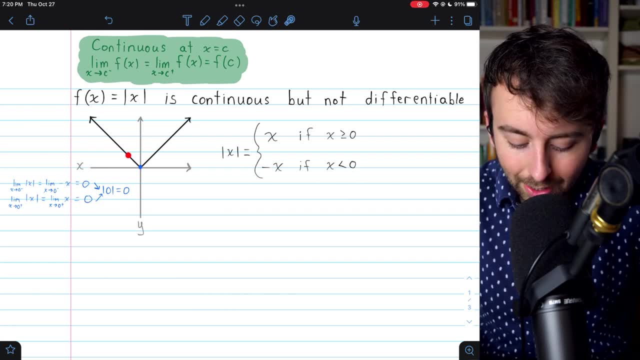 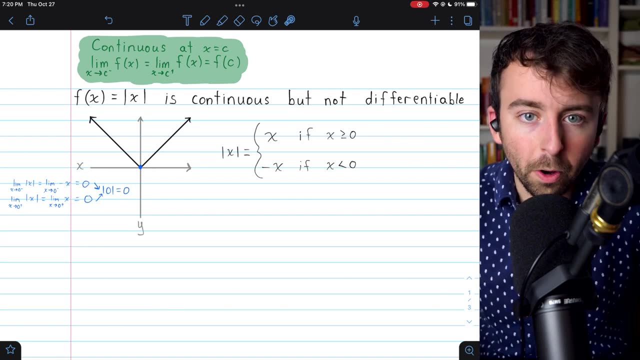 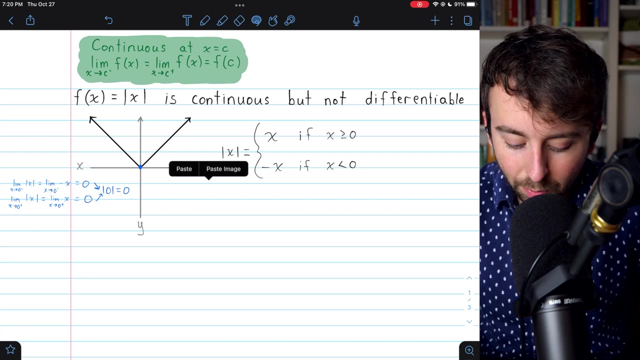 So certainly the limit of the slopes from the left and the right could not be equal, and so the derivative there will not exist. This is what we call a corner, where the derivative from the left doesn't equal the derivative from the right. But just to show that this does in fact. 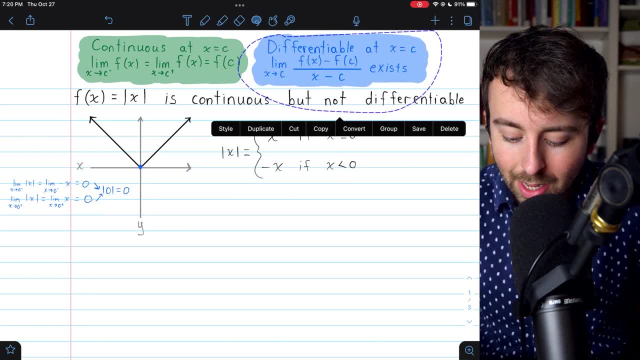 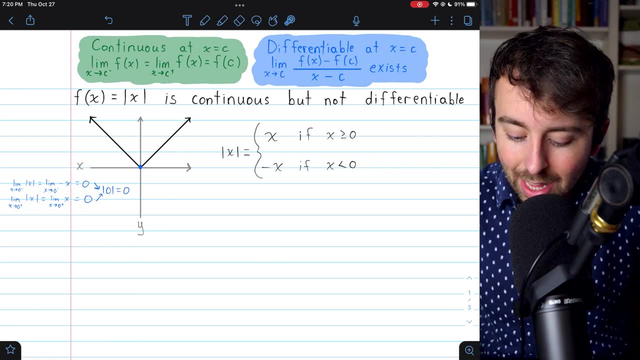 not exist this derivative. let's make sure we recall the definition of a function being differentiable at x equals c. If it's differentiable at x equals c, that would mean that the two-sided limit as x approaches c of f of x minus f of c. 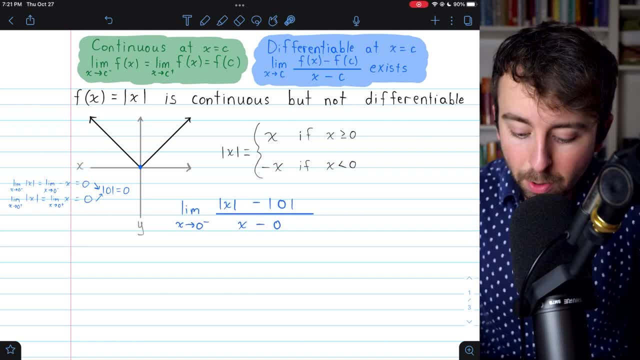 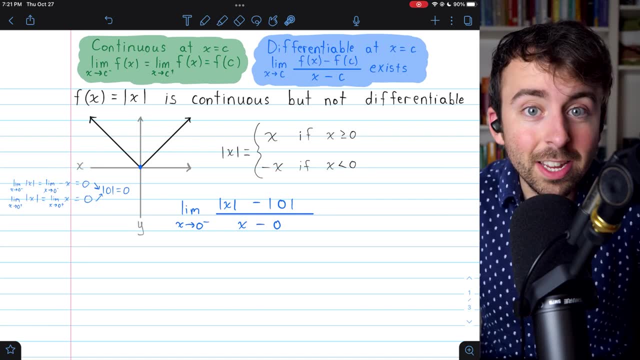 over x minus c exists. And remember this limit. expression is just the definition of the derivative. So what makes a function differentiable at x equals c? Well, it's, if the derivative at c exists, To show that this limit doesn't exist. 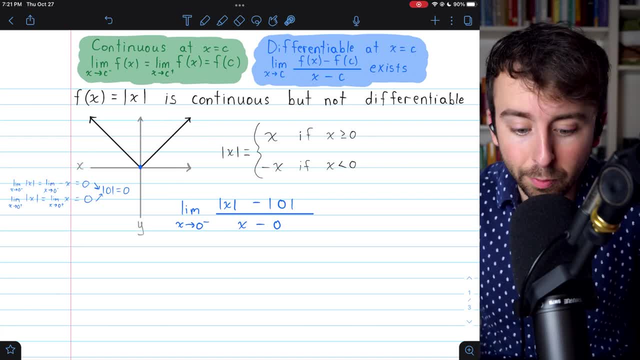 we'll evaluate the one-sided limit and show that they differ: One's negative one, the other one is positive one, which will show us that the two-sided limit defining the derivative can't exist, since the one-sided limits are different. So we begin by just taking this definition. 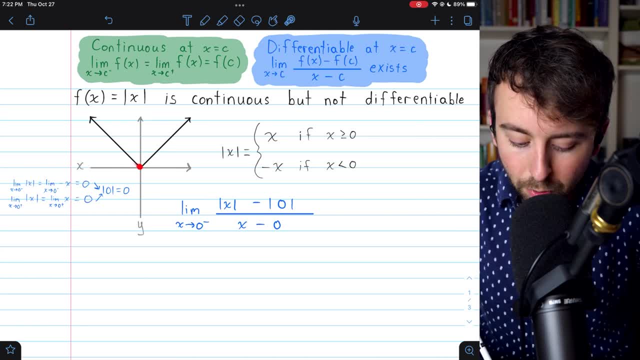 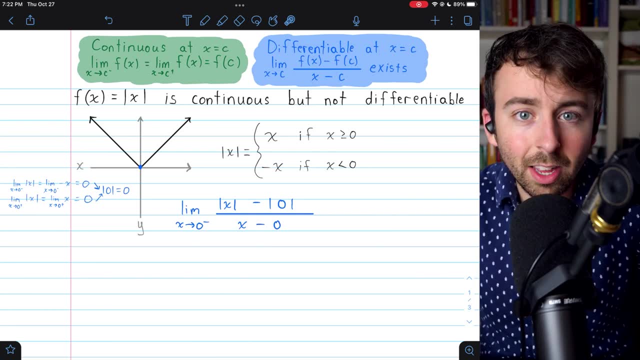 and applying it to our situation. We're looking at x approaching 0.. We'll start off with approaching 0 from the left, And again it makes sense to split this up into the individual directions, because the behavior of the absolute value function. 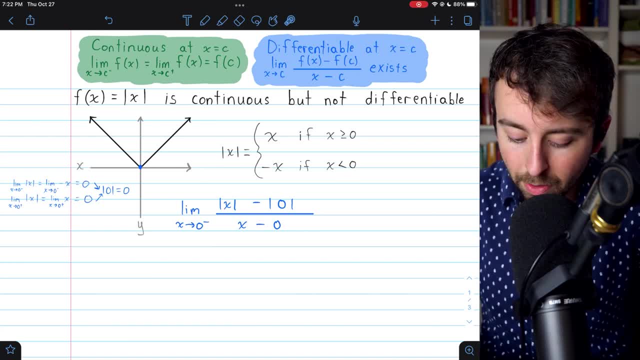 differs depending on if we are to the left of 0 or to the right of 0. So here is this expression from the derivative definition. We have our function, absolute value of x, minus our function evaluated at the point in question, evaluated at 0,. 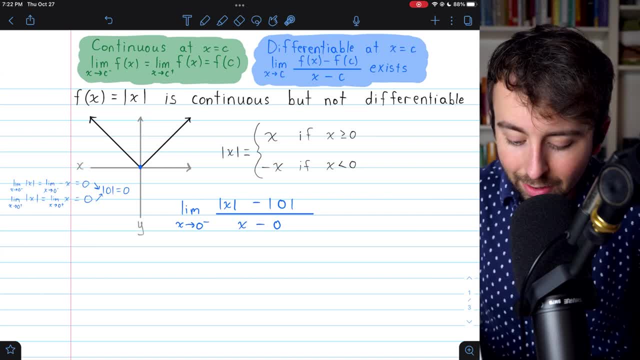 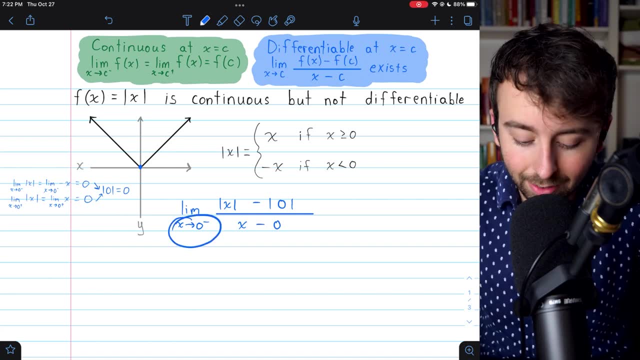 and then divide by our variable x minus the point in question. Again, that is 0. in this case. Now, since x is approaching 0 from the left, x is negative and so absolute value of x, as we've discussed, is negative x. 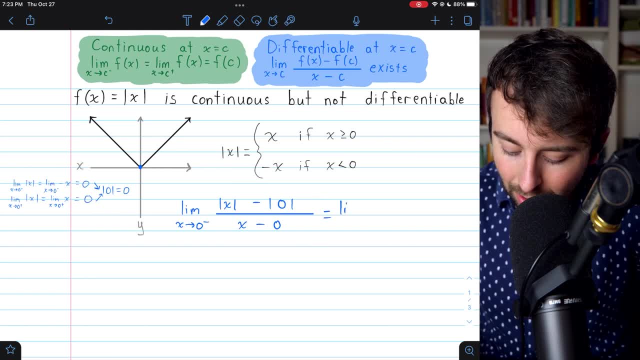 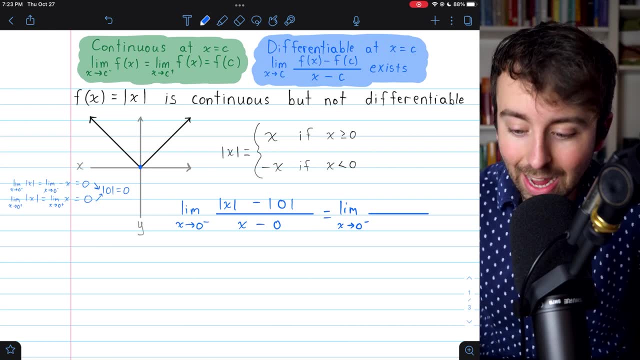 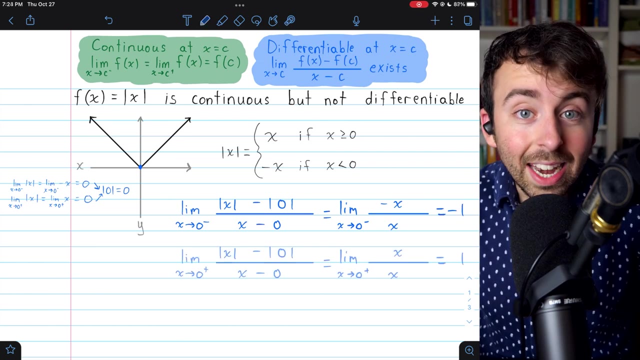 So this whole numerator is just negative x minus 0.. In the denominator we have x minus 0, which is just x. So this is negative x divided by x. As we expect, this is negative 1.. A nearly identical procedure shows us that the slope